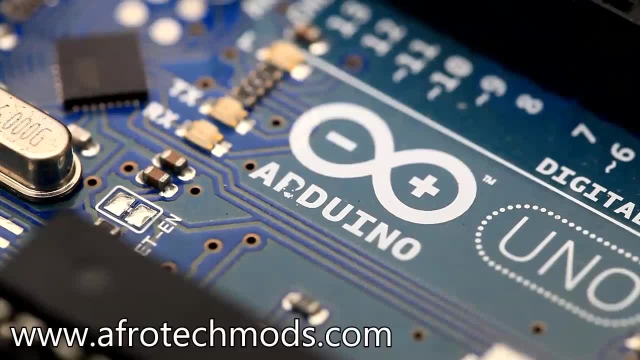 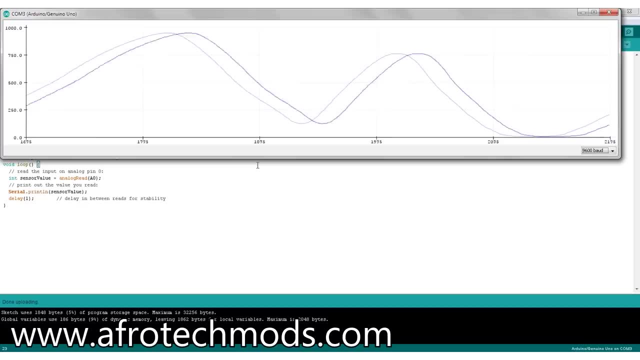 Arduinos. I'm going to talk about what they are, what they can do and the basics of how to set one up to do simple things like make an LED dimming circuit, control the speed of motors and even make a simple oscilloscope. So what is an Arduino? I'm sure you've heard about these things a million. 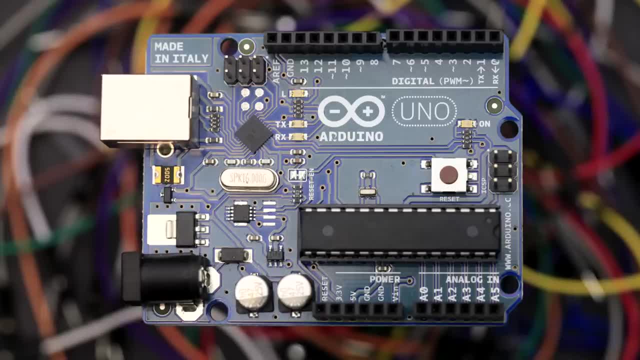 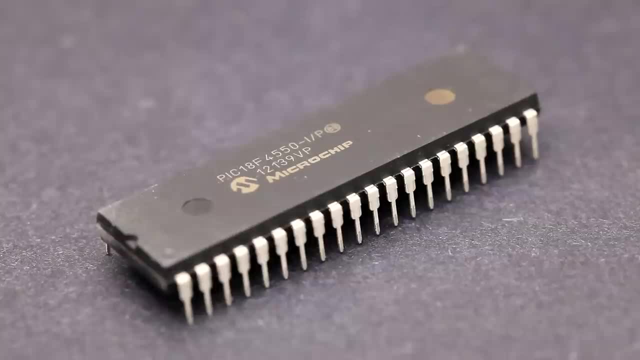 times by now, and if you're confused you have every right to be, because the word Arduino refers to so many different things. Keep watching and I'll explain all of them. Microcontrollers are integrated circuits that are basically tiny computers. They can run small, simple software. 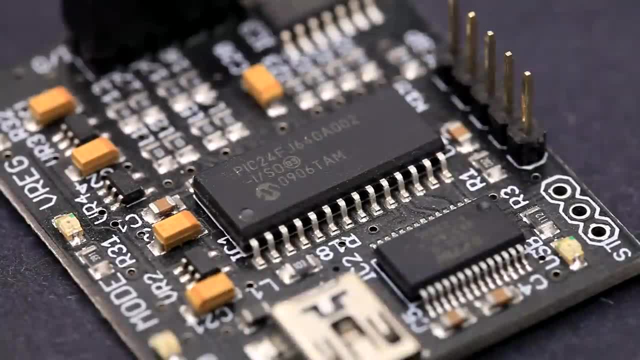 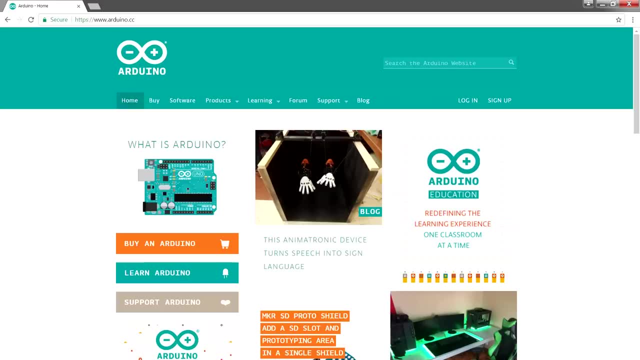 programs. They're low-powered enough that they can be powered by a battery for days, but they're fast enough to process data- much faster than any human being can think. Arduino is a company in Italy that designs and sells circuit boards that make microcontrollers. 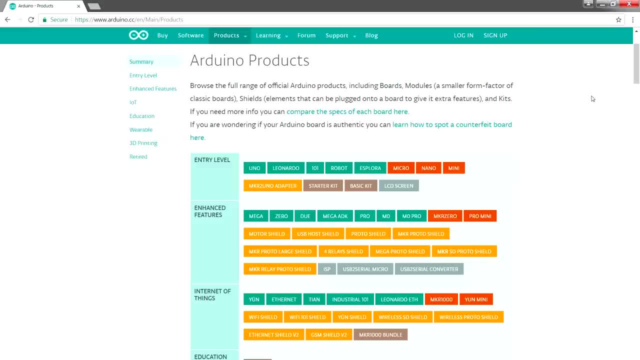 easy to use. They call these circuit boards Arduinos, and there are a lot of different types of Arduinos. For example, you've got simple Arduino boards like the Arduino Uno, which is a simple circuit board that can be used to control the speed of a computer. 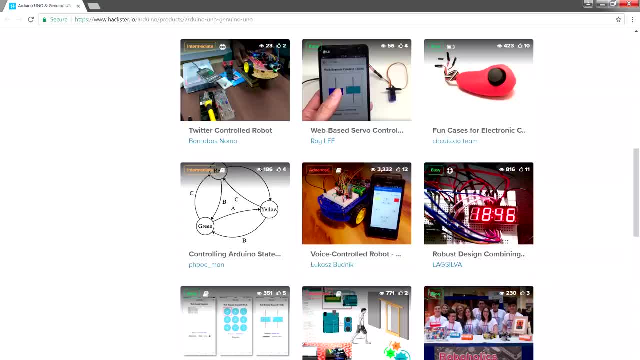 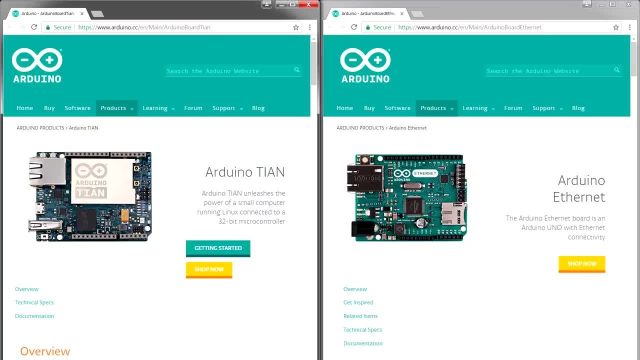 It's cheap and good enough for most projects. You could use an Arduino Uno to control motors, lighting cameras or even build a simple robot. And then you have more fancy Arduinos with more powerful processors, which have Wi-Fi, Ethernet and more. The company Arduino. 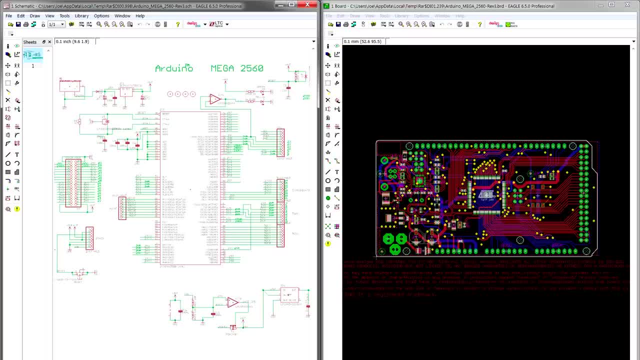 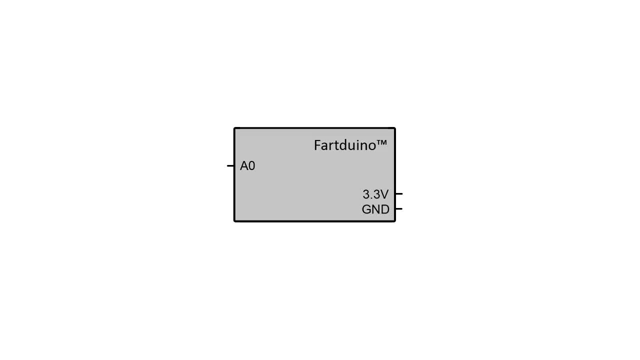 open-sources all of their hardware designs, which means that you don't just have to buy from them. There are countless third-party companies that make their own variants of the Arduino hardware designs. They can't call them Arduinos, but functionally they're. 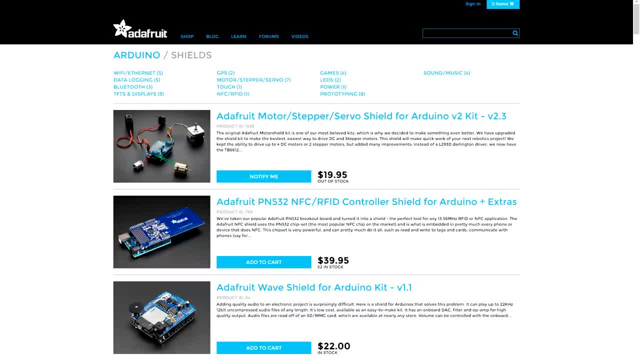 the same thing. There are also these things called Arduino shields, which are basically circuit boards that plug into your main Arduino circuit board and let you do more stuff. For example, Adafruit makes shields that let you control motors and servos without having to. 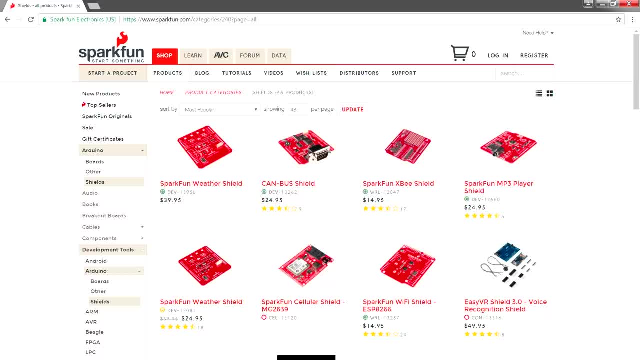 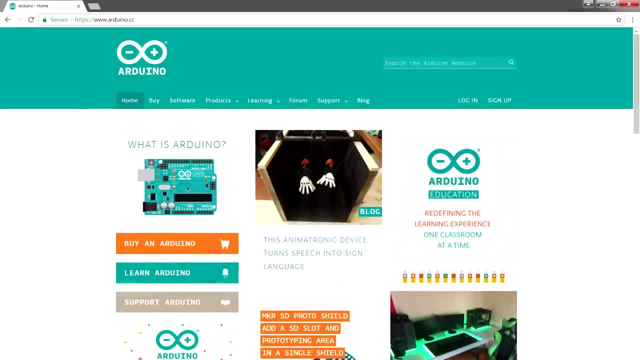 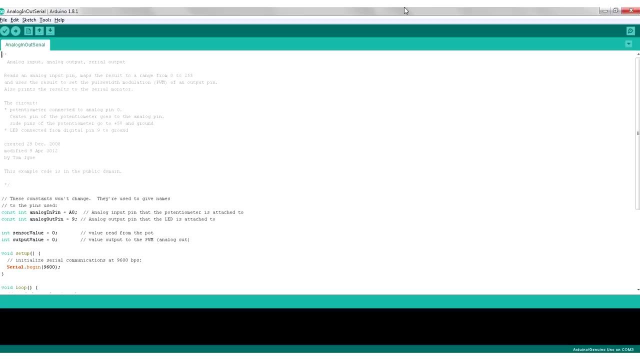 design, motor control circuitry And Sparkfun have shields that let you turn your Arduino into a simple cell phone or an mp3 player. Okay, so, that was a quick overview of Arduino, the company and Arduino hardware, but there's more. There's also the Arduino software development environment. 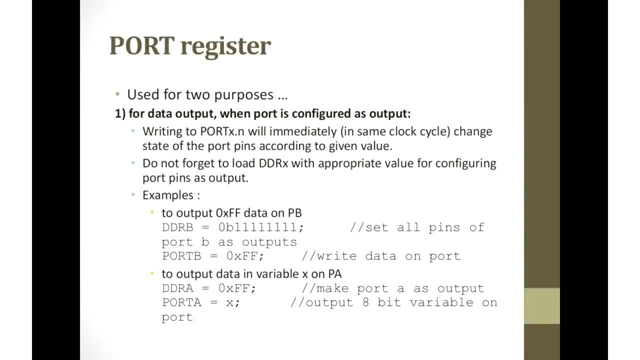 and this is what makes Arduino good for beginners. Historically, if you wanted to program micro controllers, you'd have to type out a lot of binary and memorize a lot of hard-to-remember registers and instructions. Then you'd have to use special programming hardware with custom-made 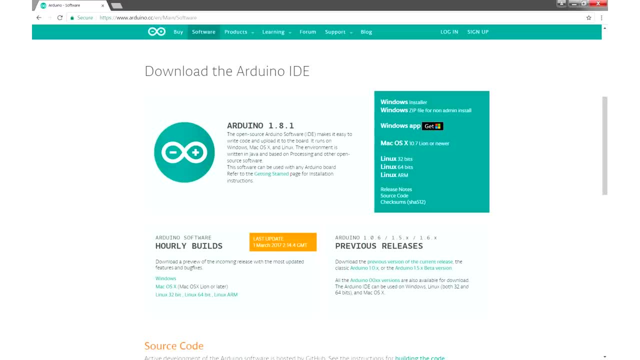 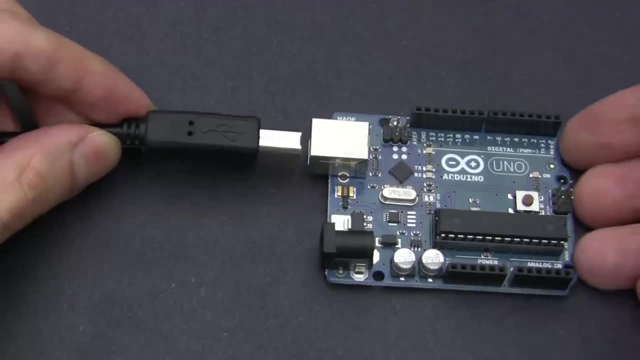 cables to upload your program onto your microcontroller, Arduino. the company got rid of all of that. They created software that works on Windows, Mac and Linux, which makes uploading as simple as connecting a USB cable and clicking a button. They created a programming language. 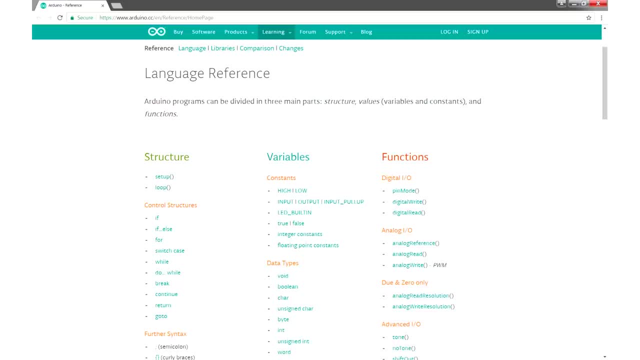 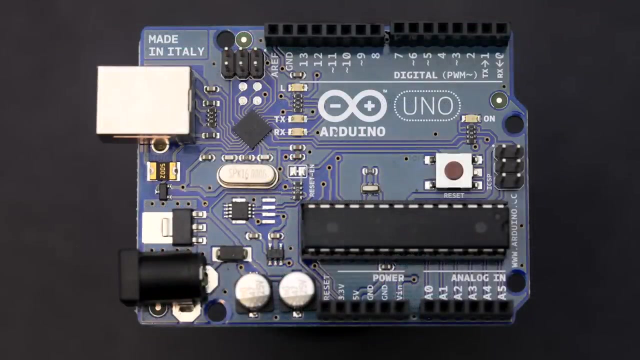 that lets you configure all of the Arduino hardware products in the same way, And, although it's not as simple as learning Python, the Arduino software is one of the easiest programming experiences you'll ever have. Okay, so hopefully that clarifies what Arduino means in different contexts. Now, when people 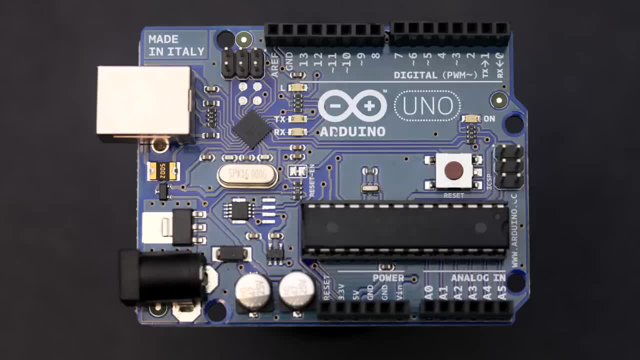 say they used an Arduino for their project. they're probably talking about the Arduino Uno. It's highly unlikely that you'll outgrow one anytime soon, so it's the perfect Arduino hardware for this beginner's tutorial. You can get them from Amazon cheaply and if you have the 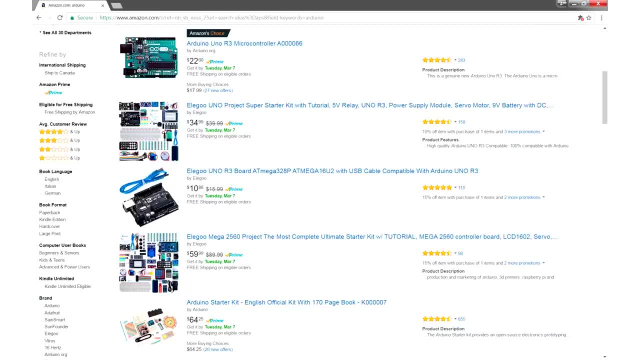 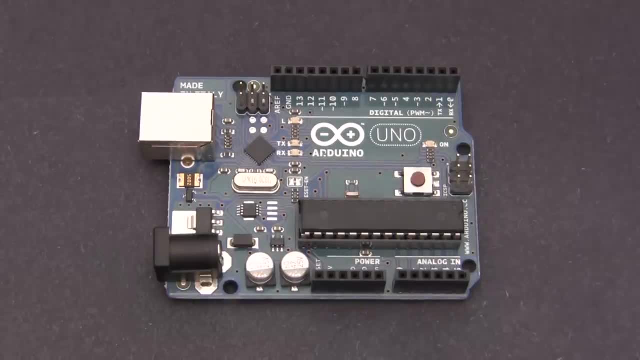 money, I recommend buying one of the many Uno kits out there, where you get a lot of different pieces of hardware to play with. Okay, so you've got your Arduino Uno. The first thing I want to do is get you familiar with the hardware. You'll often hear Arduinos being called microcontrollers. 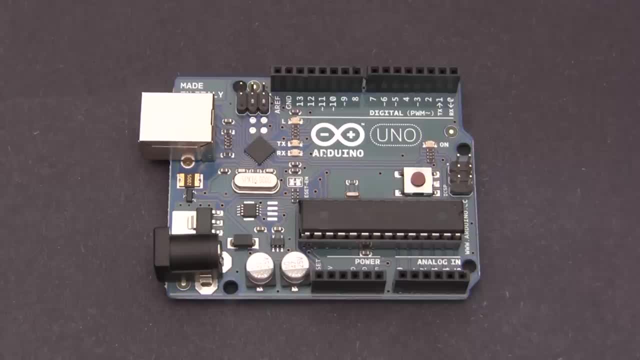 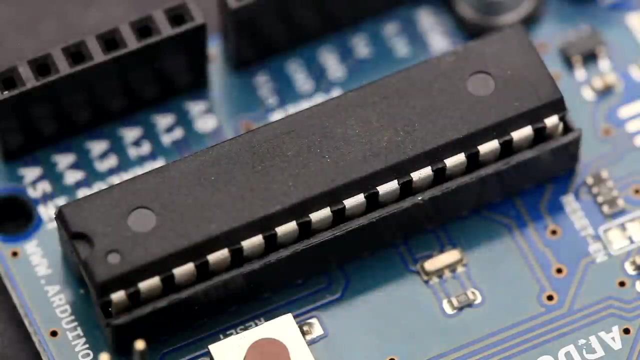 and that's technically incorrect. Arduinos are circuit boards that have microcontroller chips on them, but they also have a lot of other stuff on there too. Let's take a quick tour. This is the microcontroller Arduino. Unos use a series of microcontrollers called Atmega AVRs. They're made by a company called Atmel. You can buy just the bare chips on their own for about a dollar, but then you'd have to do a lot of soldering. Connected to the microcontroller is a crystal resonator. This controls how fast the microcontroller is running. I have a separate 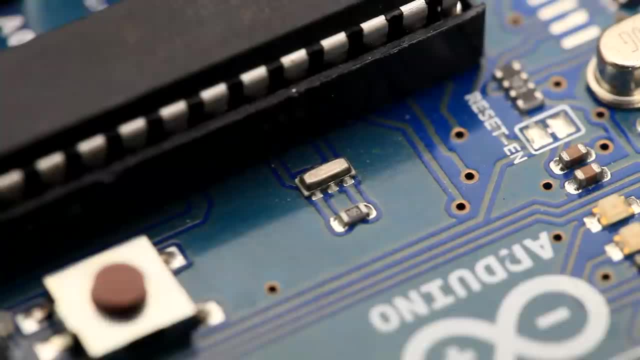 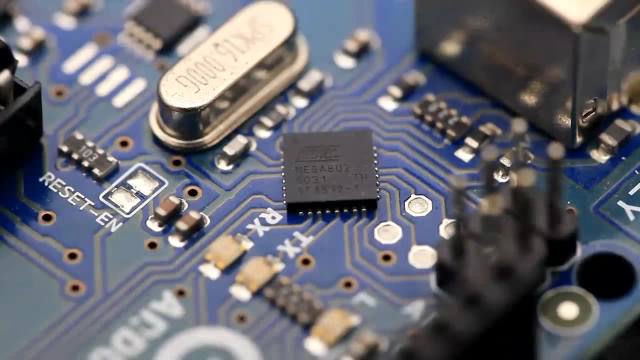 tutorial on resonators and oscillators in the description below. If you're interested in learning more about resonators and oscillators, you might find this tutorial useful. Now, in order to upload the software you create to the main microcontroller, there's actually another microcontroller. This chip is what lets you connect your USB. 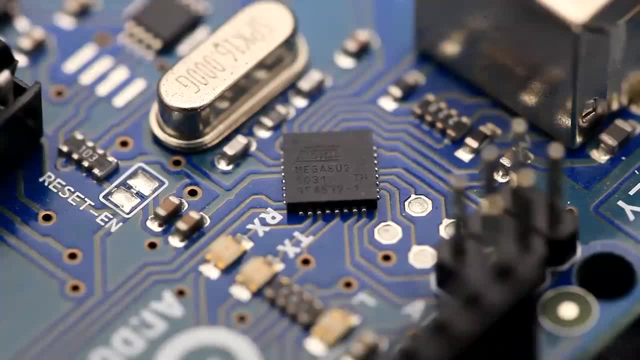 cable to the Arduino board and communicate via USB. It lets you upload your programs onto the main microcontroller and once you have your program running, this chip is what allows you to send messages back and forth between your computer and your Arduino, and this is extremely. 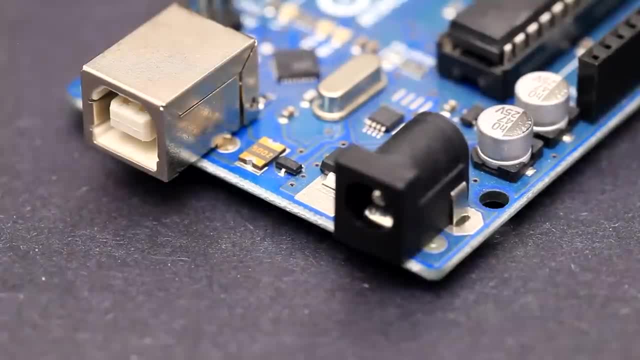 important for debugging. This chip allows you to send messages back and forth between your computer and your Arduino, and this is extremely important for debugging. One great thing about this chip is that you can power them purely from your USB cable. But if you don't want your project? 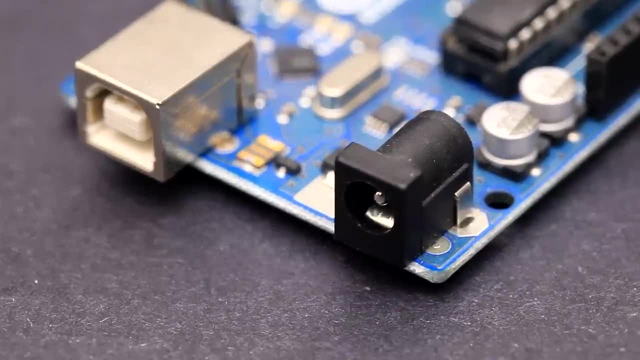 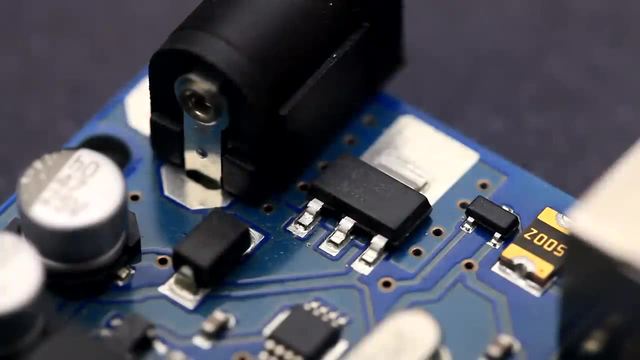 always attached to a computer. you can just use an external 9 volt DC power source with a barrel jack over here. The Uno has a built-in voltage regulator that'll reduce the voltage to 5 volts, And if you ever want to reboot your Arduino's program, you've got a reset button. 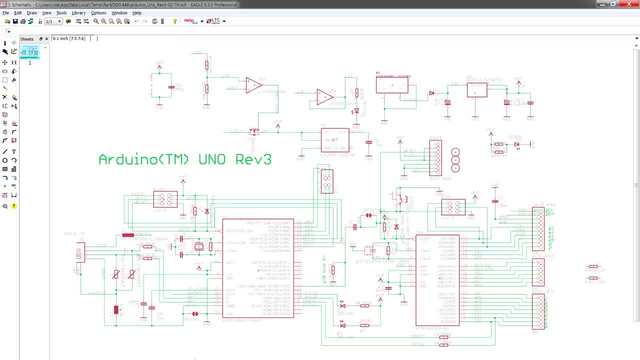 If you have time, it's worth studying the Arduino Uno schematic. Don't worry if it looks complicated. You don't need to understand most of it. I'm just trying to get you to understand what the Arduino designers did. They took an off-the-shelf. 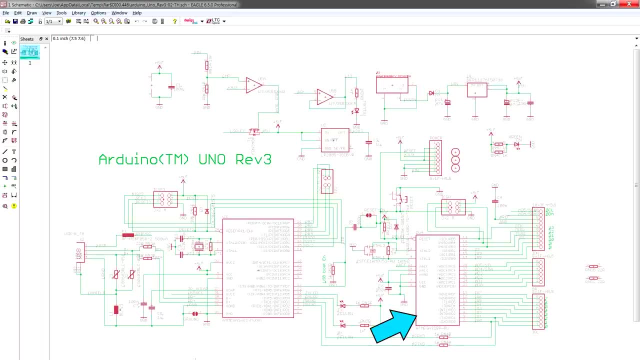 microcontroller. that requires a lot of extra parts to get working, and they put all of those things together in an easy-to-use way, And if you choose to learn more about electronics, you can create circuit boards like this too. Okay, so that's what's under the hood. Next, let's talk about 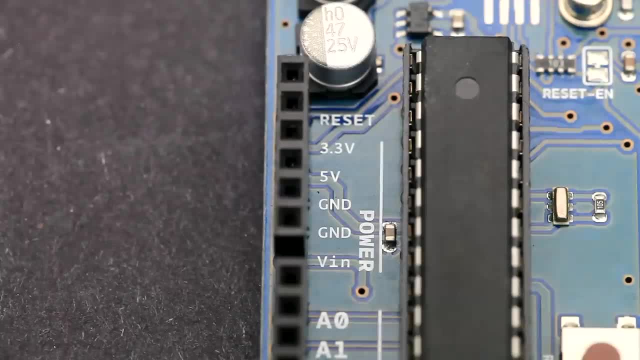 the pin connectors. Over here you have the power pins. If you want, you can connect wires here to other circuitry with 5 volts or 3.3 volts. That's all there is to it. Just make sure that you're that whatever you power doesn't draw more than a few milliamps. A few LEDs is ok, but 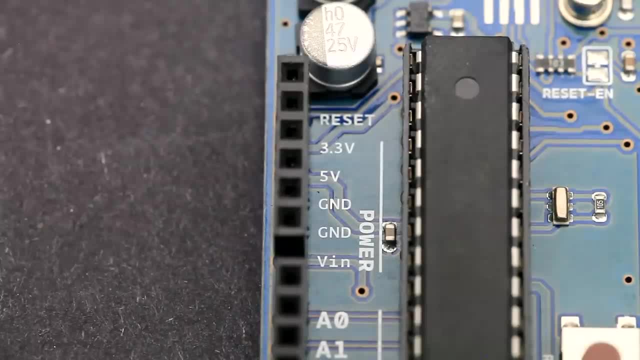 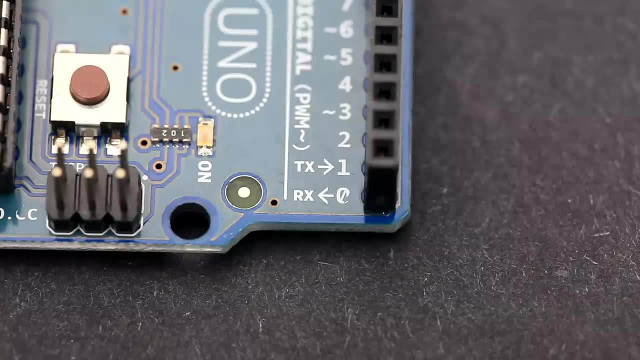 a large motor would be an arduinono. Boo, You suck TX. and RX is for sending and receiving serial data. You could use this port to send and receive data from a GPS module, bluetooth modules, wifi modules and more. 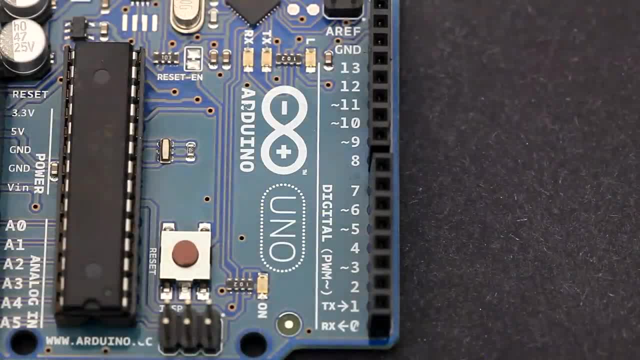 Pins 2 to 13 are for digital inputs and outputs. Normally when people think of binary, you think of just spitting out 0s and 1s, But with most microcontroller pins you can actually activate a third state and use them as a digital input. So you can use this pin as an output where 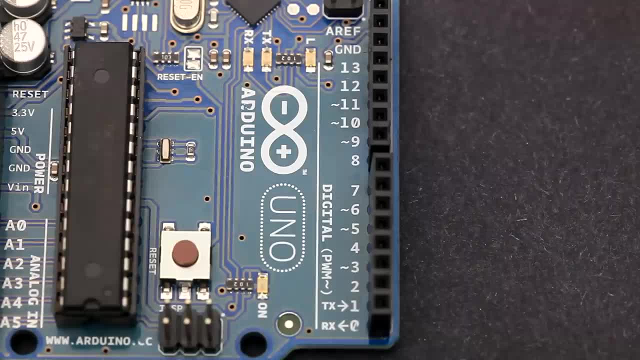 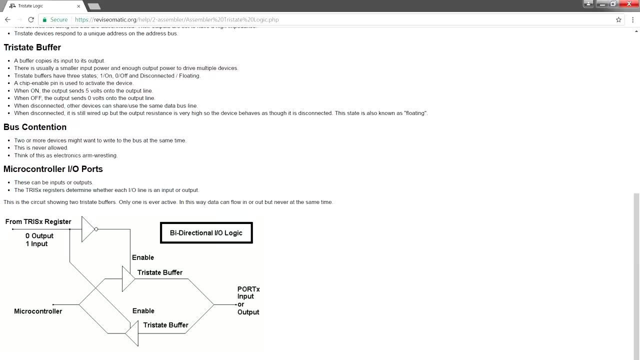 it spits out 5 volts for a digital 1, or 0 volts for a digital 0, or you can internally configure the arduino to expect a voltage on the pin and that voltage could be interpreted as a 1 or a 0. It's a system called tri-state logic and it's worth reading up on. but 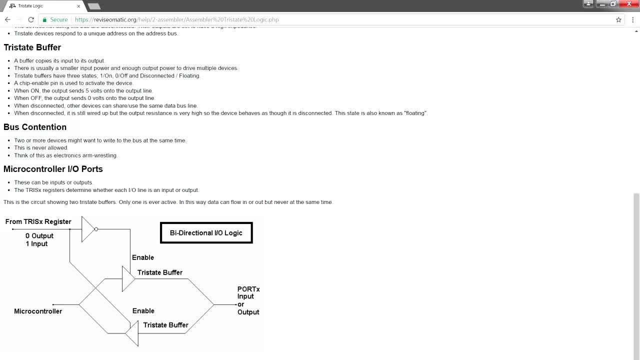 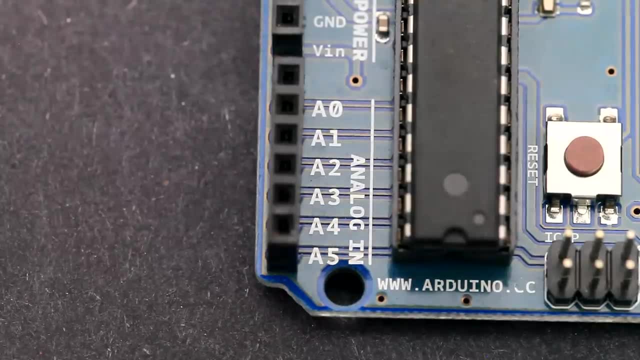 arduino makes it really easy to change between inputs and outputs in software. Here we have 6 analog input pins and these are used to measure continuous voltages anywhere from 0 volts to 5 volts. I'll talk more about this later in the video. 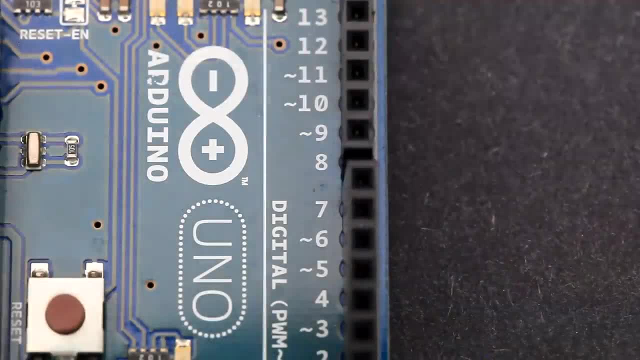 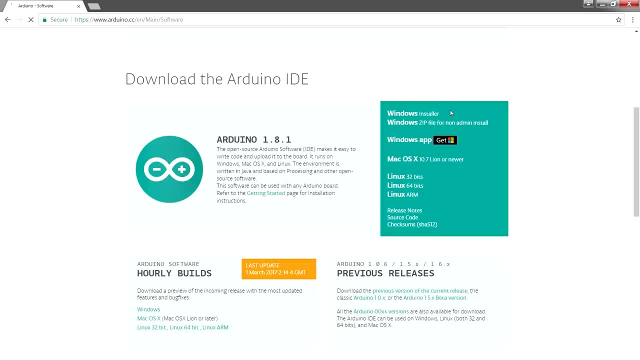 Finally, some of the pins have a tilde in front of them, and this means that you can use them to output pulse width modulated square waves, which I'll also show later in the video. Ok, enough about the hardware. Most of the work you do with your arduino is just to make sure that you're getting the 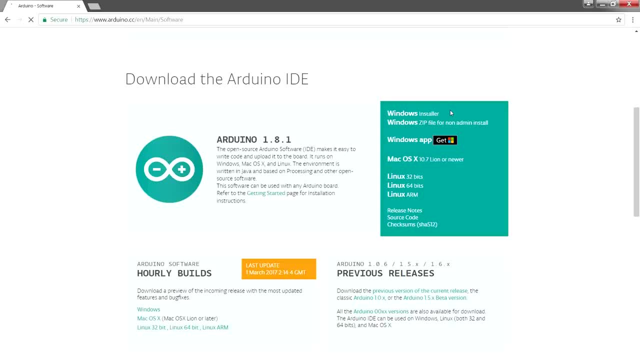 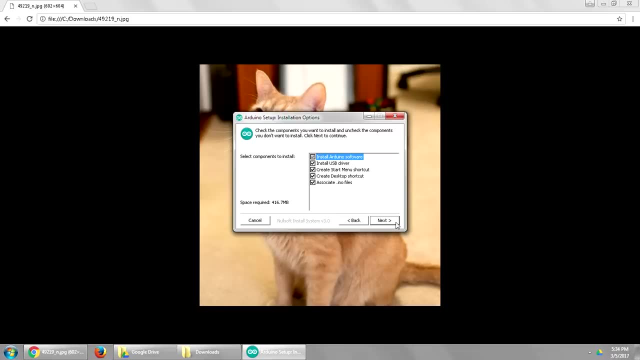 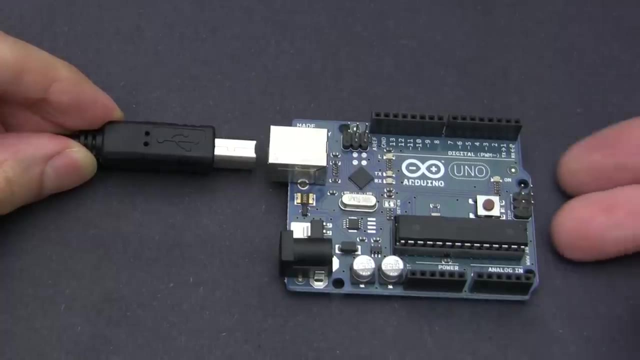 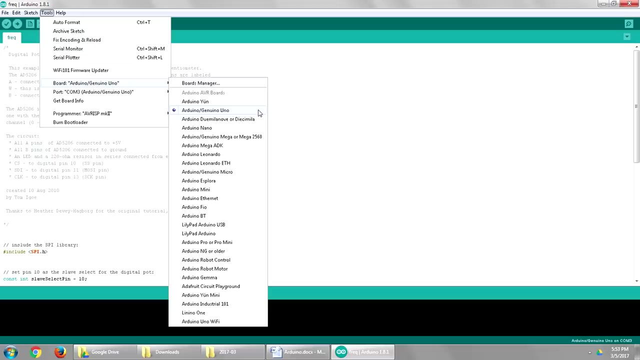 most out of it. The first thing you want to do is make sure that the software tries to connect to the right type of arduino. Go to tools boards and we're going to be using an arduino uno. Next we have to make sure that the arduino environment can actually connect and communicate. 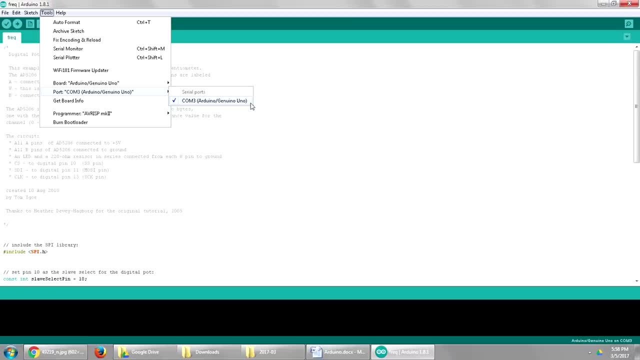 with your arduino. Go to tools ports and select the com or serial port where your arduino is connected. If there isn't an arduino listed here, you may have a problem with your drivers, or you can try plugging your arduino into a different USB port. 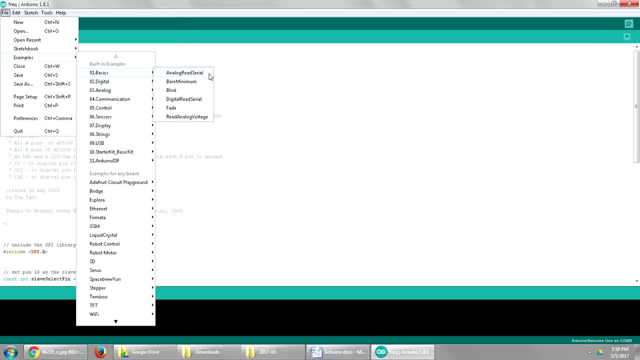 The arduino software has a ton of fantastic, easy to follow demo programs and it's a great way to connect your arduino to your arduino. Arduino calls them sketches, which is just a fancy name for a program that you upload to your arduino. 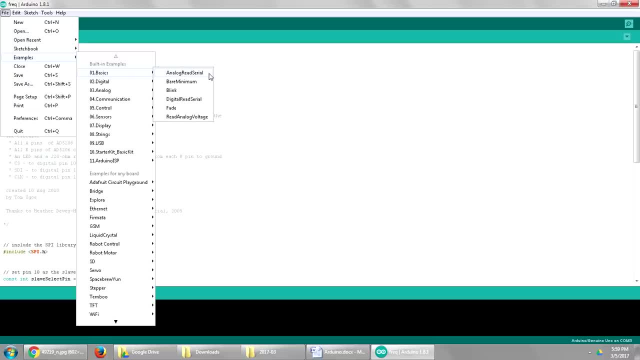 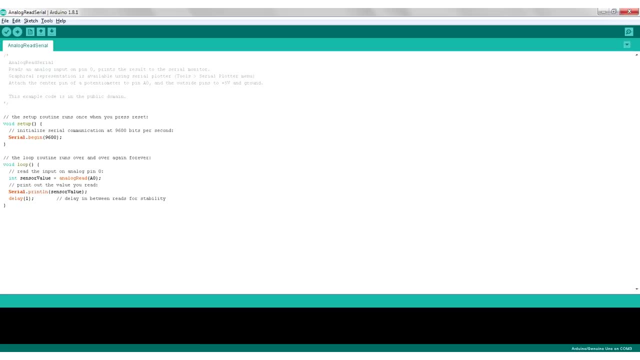 Let's start with an example where we measure voltages that are being fed into the arduino. Go to file examples. basics- analog, read serial. All the arduino examples contain instructions on how to set up the hardware. This one is telling us attach the center pin of a potentiometer to pin A0, and the 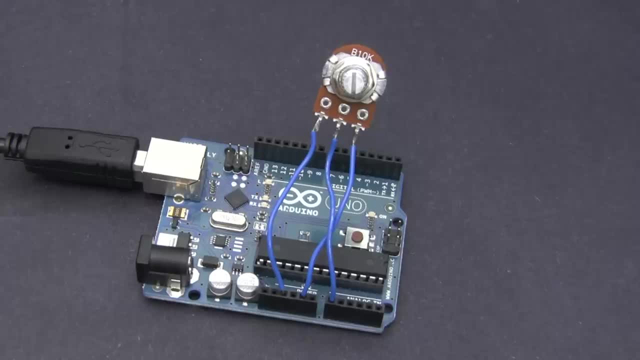 outside pins to plus 5 volts and ground. Ok, let's do that. A 1k or a 10k potentiometer will work great for this. We're going to be using it as a voltage divider to create a voltage anywhere from 0 to 5 volts. 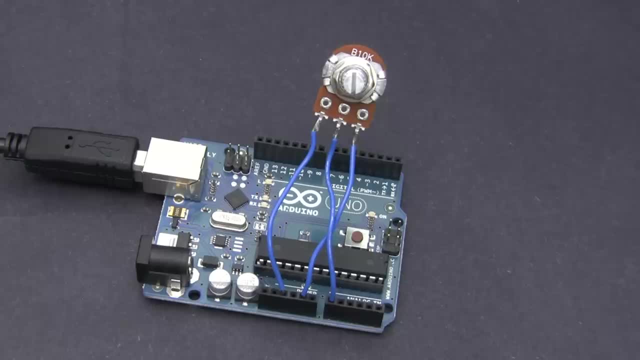 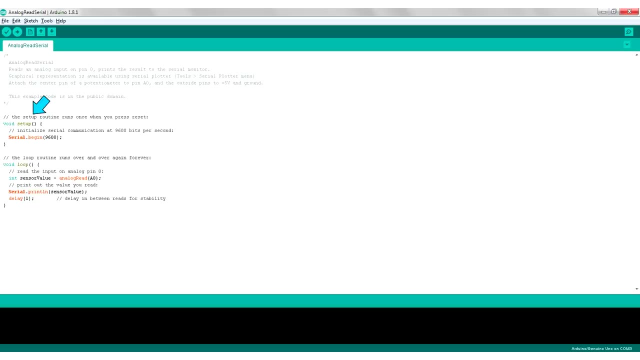 Make sure you've watched my voltage divider tutorial if you don't understand how that works. Every arduino program will have two main areas: the setup and the loop. The setup area is where you configure your arduino to do certain things for the duration. 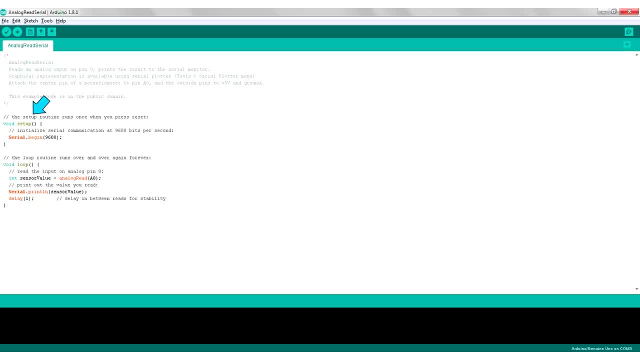 of your program. This can be information on which pins are inputs and which are outputs, but in this case we're telling it to send serial data to our computer at 9600 bits per second, which is a pretty standard data rate for these situations. 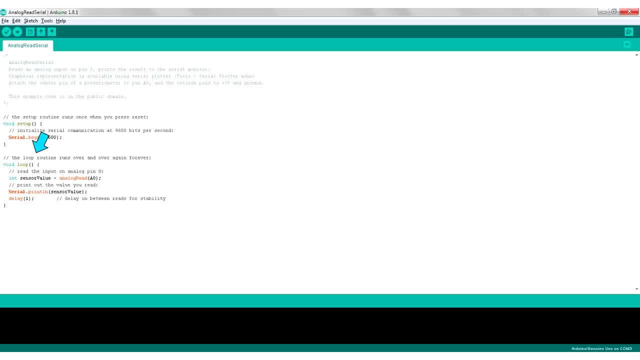 The loop is the area of code that repeats over and over again for as long as the arduino has power to it. This line will measure the voltage on pin A0 and store the value of it in a temporary place in memory that we're calling sensor value. 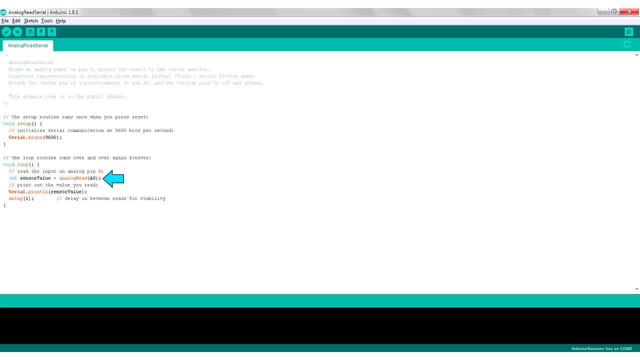 Sensor value is an int or integer. Sensor value is an integer Meaning it's a whole number. Once we've copied the analog voltage reading to sensor value, the command SerialPrincline will transmit that value from our arduino through the USB cable to our computer. and 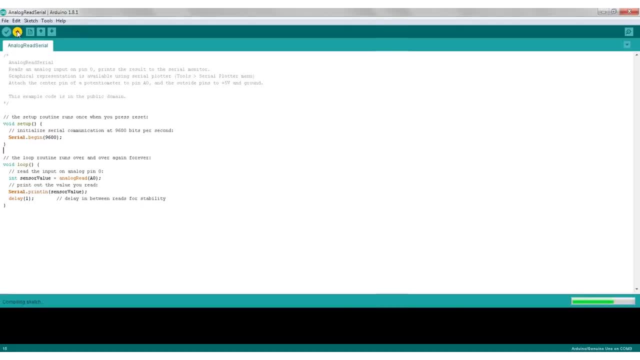 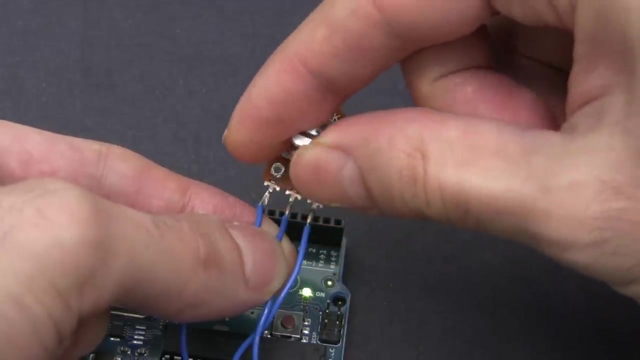 we can view it. Click upload. it will compile a sketch and upload it to your arduino. Now hit the reset button. Next go to Tools, Serial Monitor. It should see a bunch of numbers flying by. You shouldiene it potentiometer from 0 to 5 volts. you should see a number on screen from 0 to 1023. 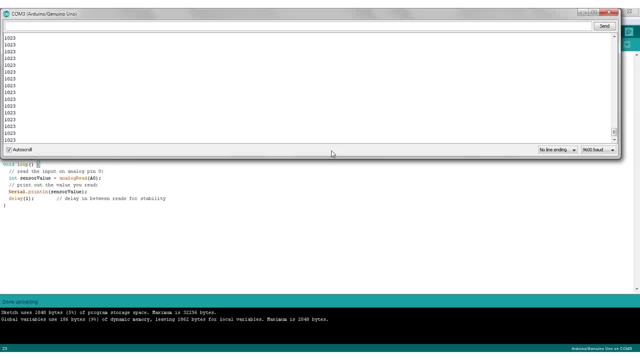 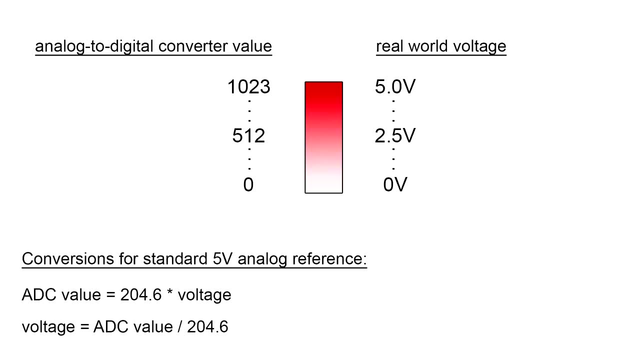 This is because internally, the Arduino represents the analog voltages it measures with a 10 bit number, which can be from 0 to 1023.. The number scales linearly with the voltage, so 2.5 volts would be halfway down at 512.. 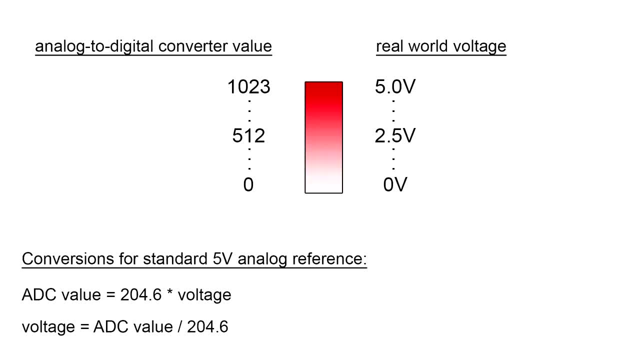 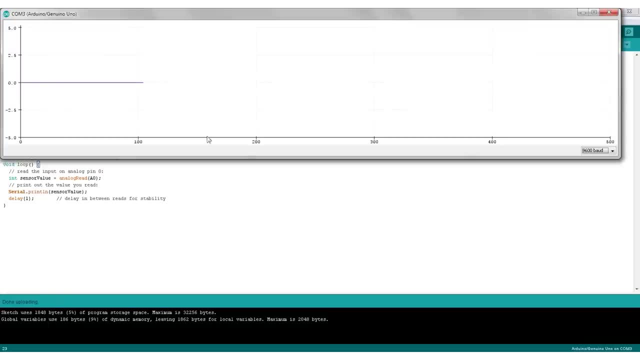 You can use these formulas to convert from analog tick values to real world voltages and vice versa. Now close the serial monitor and go to Tools- Serial Plotter. Now you can get a graph of the voltage your potentiometer is creating over time. 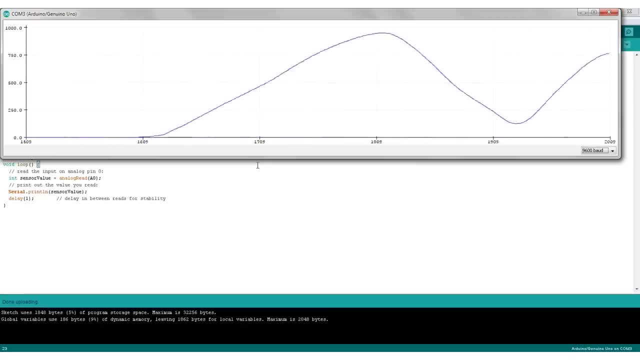 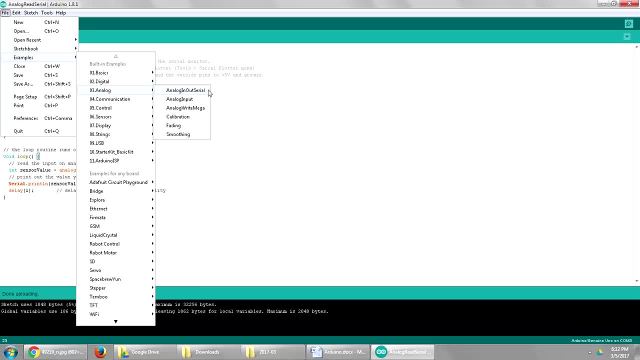 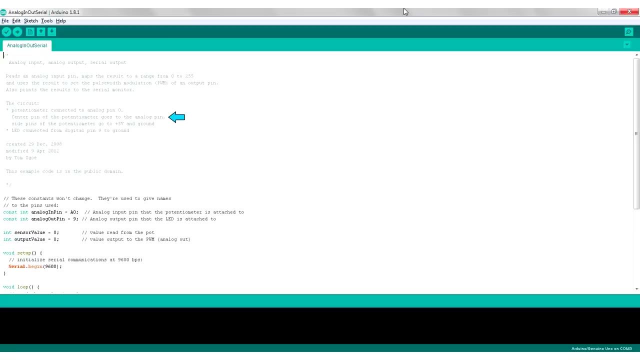 It's basically a very simple low bandwidth oscilloscope. Let's try another experiment where we build a simple LED dimmer. Go to File Examples: Analog: Analog In Out Serial. The instructions for the potentiometer are the same as before. It also says to connect an LED from digital pin 9 to ground. 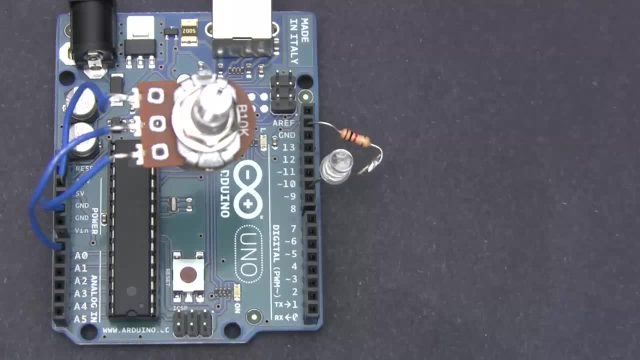 Note that it is implied that you will put a resistor in series with the LED. The pins on an Arduino can't supply much current, Any more than about 20 milliamps, and you risk permanently destroying that pin. I have detailed tutorials on LEDs and resistor values, but for now let's just use a 1K resistor. 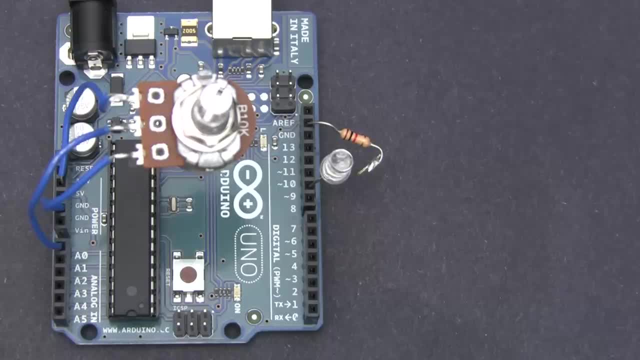 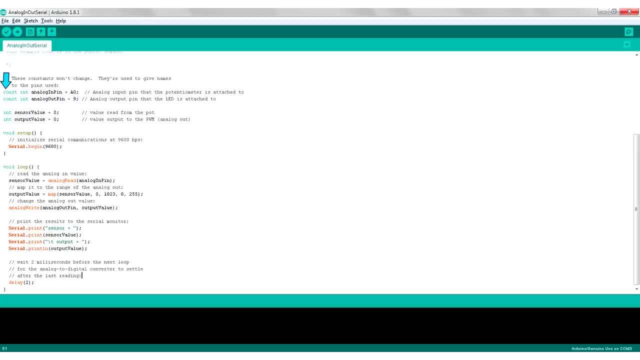 attached to ground, The other side goes to the cathode of an LED and the LED's anode goes to pin 9.. We've already talked about this. We've already talked about what an int is, But this const int means that the label analog outpin will always translate to the number. 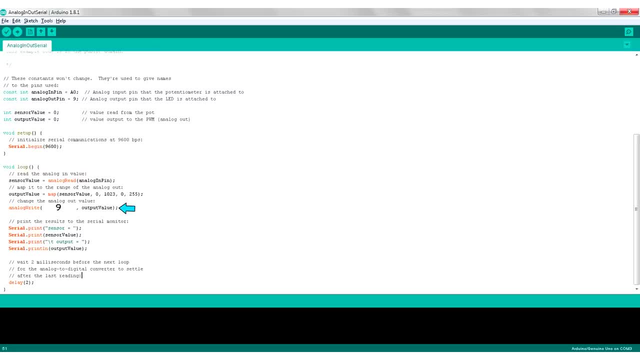 9 throughout the rest of the program. For example, here saying analogWrite 9 comma output value wouldn't be very clear. Like what the hell is the 9 for? Instead, we're declaring analog outpin to be a place in the Arduino's memory that always. 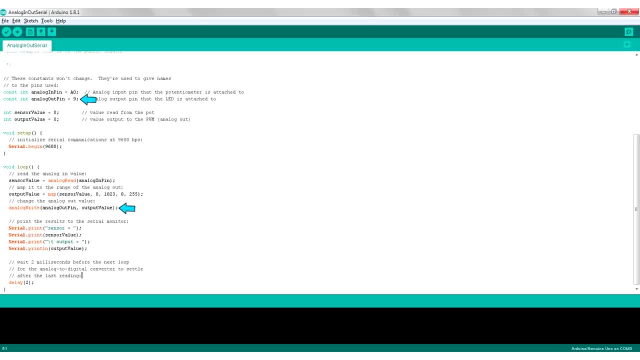 stores the fixed constant number 9.. So when we write other pieces of code, we don't have to memorize the number 9.. We don't have to memorize the constant number 9.. So when we write other pieces of code, we don't have to memorize the constant number 9.. 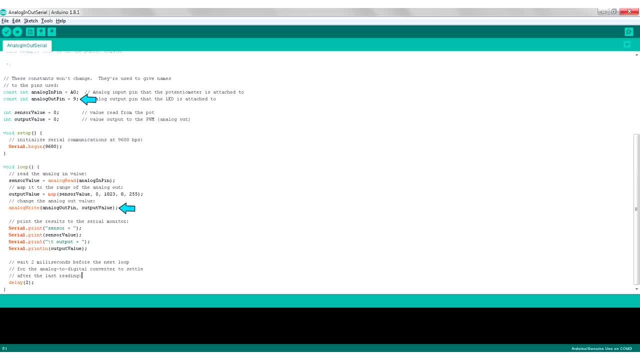 which pin numbers we're using for different things. It's not a big deal right now, but this becomes more important when we have programs that use a lot of different pins. Sensor value and output value are non-constant integer numbers, which means they can change value during the operation of the. 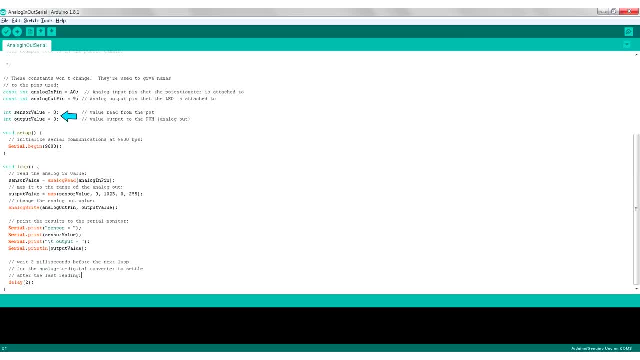 program. The term for this in programming is a variable On the Arduino platform. an int variable can hold a number anywhere between minus 32,768 and plus 32,767.. The setup is the same as before and once again we're using the analog. 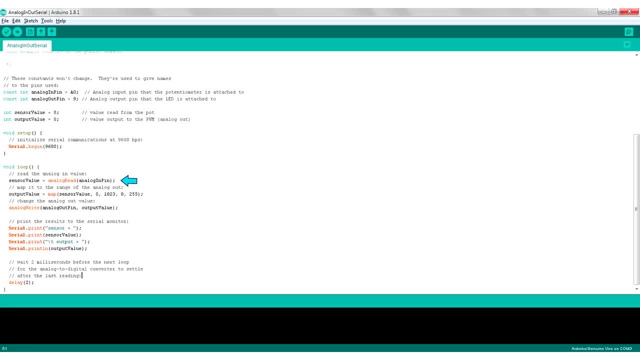 read function to measure the voltage on a certain pin, which turns out to be pin A0. We store that value in sensor value. Now we know that the Arduino internally represents analog voltages with numbers from 0 to 1023, but the analog write. 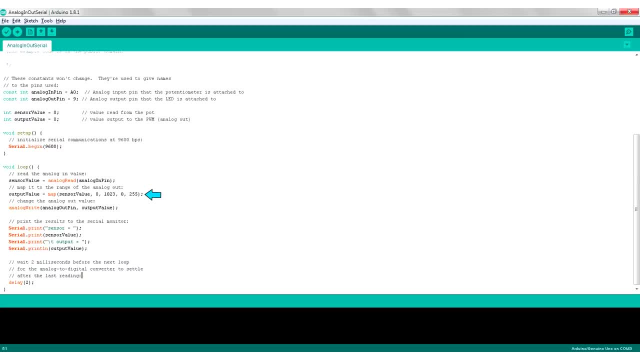 function only accepts values from 0 to 255, so we use the map function to measure the output value from the pin A0 to the pin A0.. here to linearly scale sensor value down to values between 0 and 255. Then the analog write function takes the number stored in output value and uses it to control. 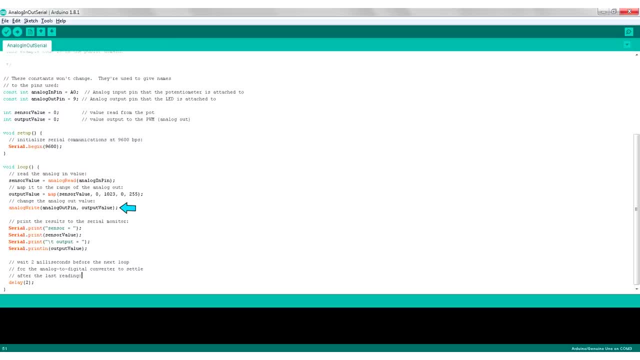 the voltage on analog output pin, which is in fact pin number 9.. The serial printing stuff is similar to what we had before, and at the end of each loop the delay function will make the Arduino pause execution of all code for a specific number. 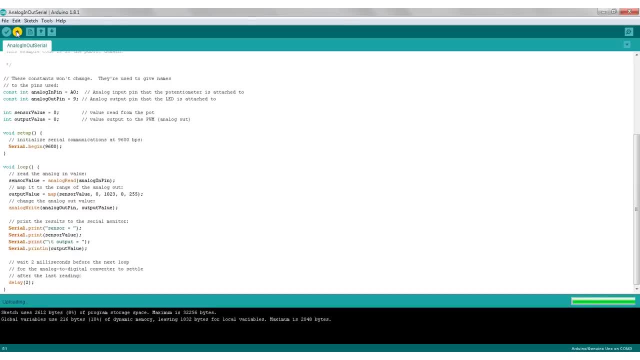 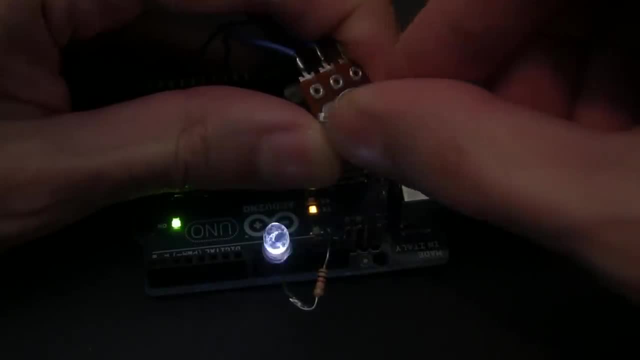 of milliseconds. Once again, we click upload, hit reset on the Arduino and now we have a system that can control the brightness of an LED with a potentiometer. Now you're probably thinking: so what? You can do that without the Arduino. 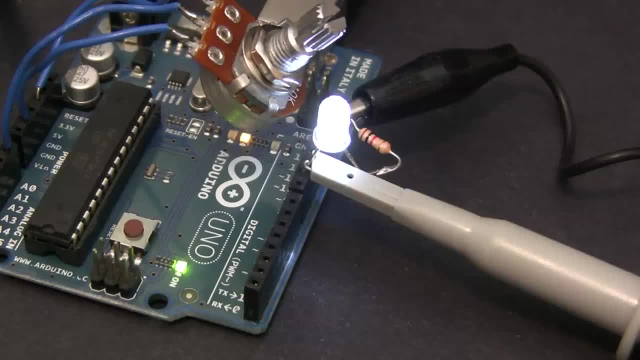 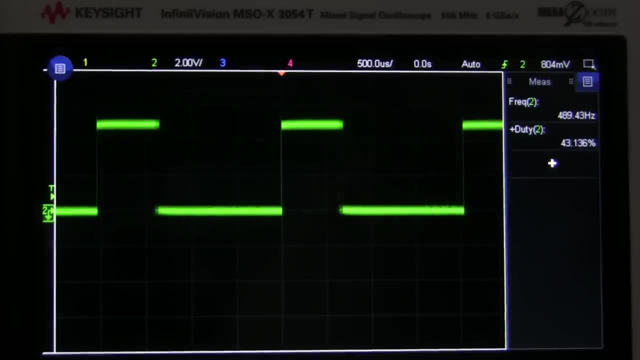 Well, let's probe the output of pin 9 with an oscilloscope to see what's really happening. here We've got a pulse width modulated square wave. We can control it with a potentiometer, and it's very precise. Now, instead of an LED, let's control something else. 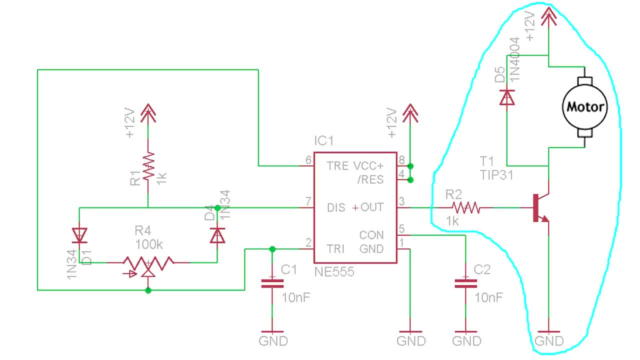 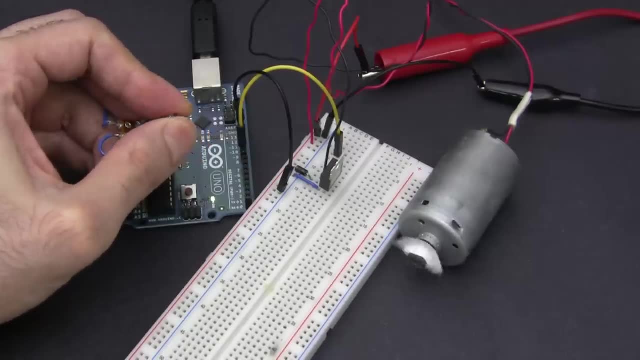 Let's take this part of the circuit from my classic pulse width modulation tutorial, and now we'll be able to control a motor digitally instead of a sometimes glitchy 555 circuit. So you might be thinking that it's weird that an Arduino function called analog write is. 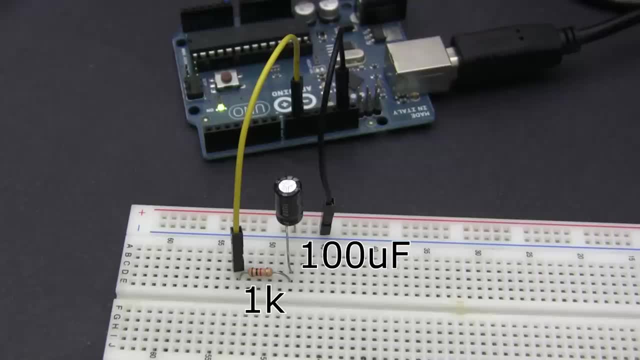 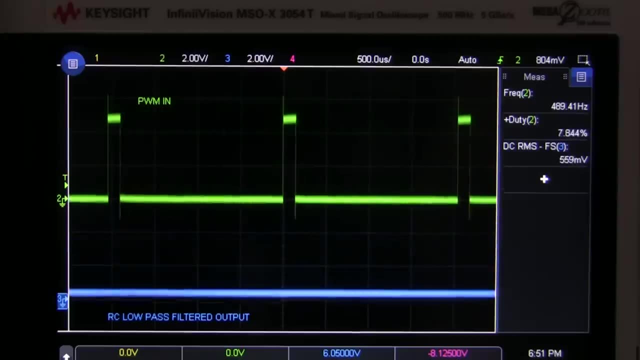 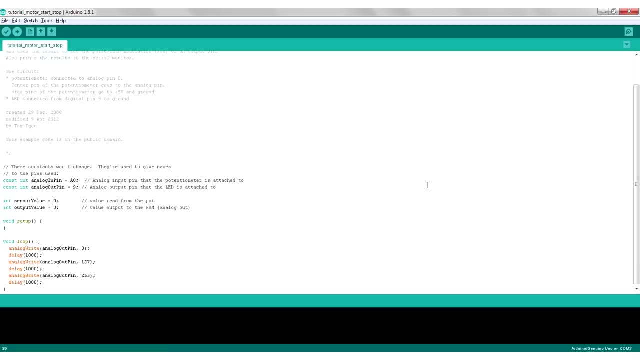 in fact controlling a pulse width modulated square wave. Well, the idea is that you would use an RC low pass filter to convert that square wave into a continuous analog voltage, and I have separate tutorials on how to do this. Once you've looked at a few examples and understand how they work, you can delete pieces of code. 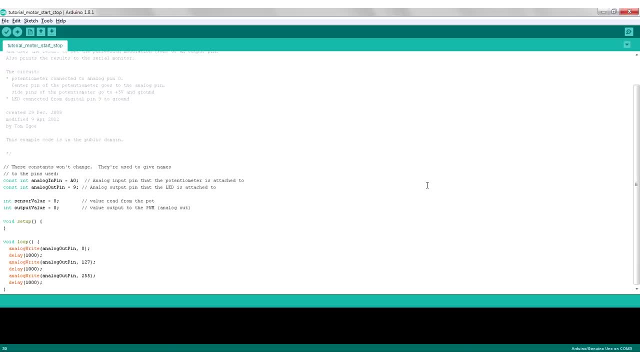 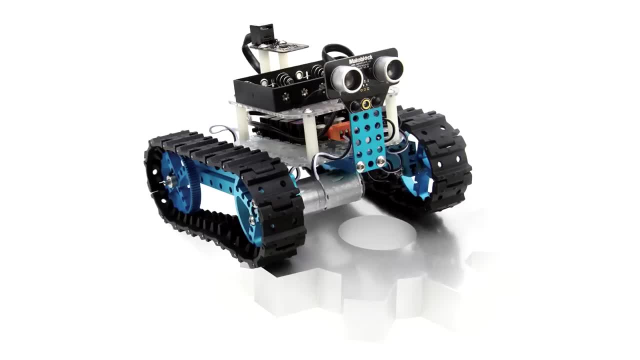 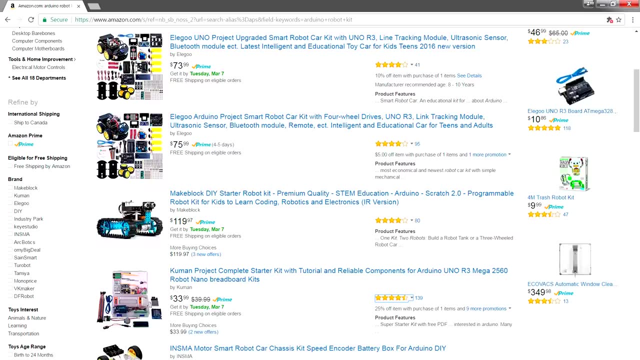 So you can see how, by reading voltages from sensors and writing code to control motors and servos, an Arduino can easily become the brains of a simple robot. In fact, you can get kits to build Arduino based robots for as little as $74.. 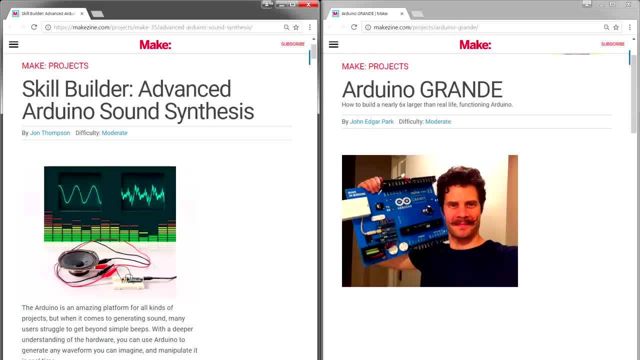 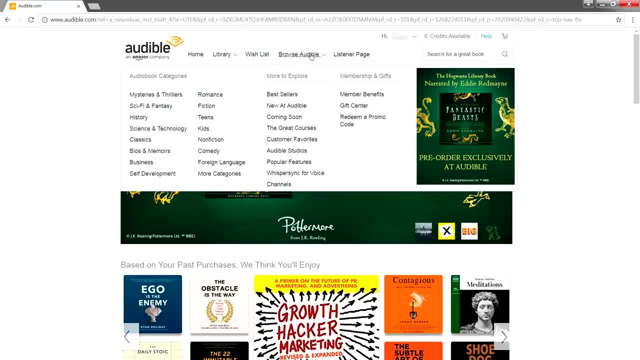 So those were just two easy examples of what you can do with an Arduino, but you can do so much more and there are tutorials all over the internet for them. Thank you for watching and if you found this video useful, please check out my sponsor, Audible. 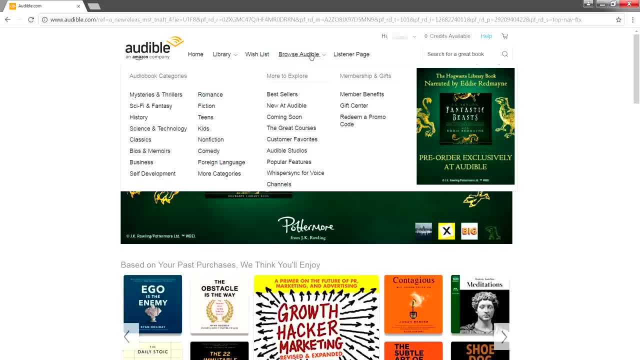 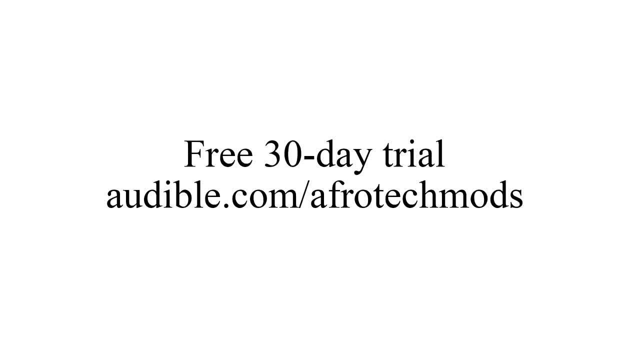 Audible is a company owned by Amazon and basically they have a huge selection of audiobooks that you can buy and listen to on the way to work or when you're at the gym. They've got a promotion right now where you can get a free audiobook if you sign up for. 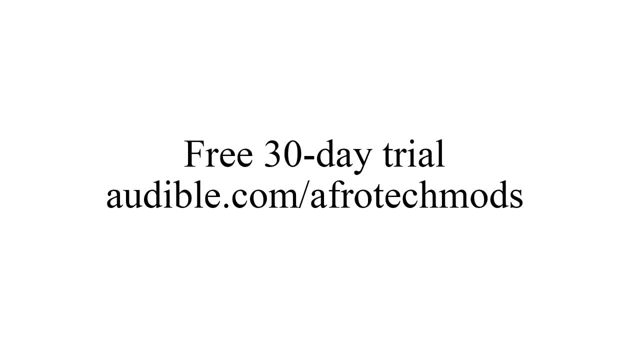 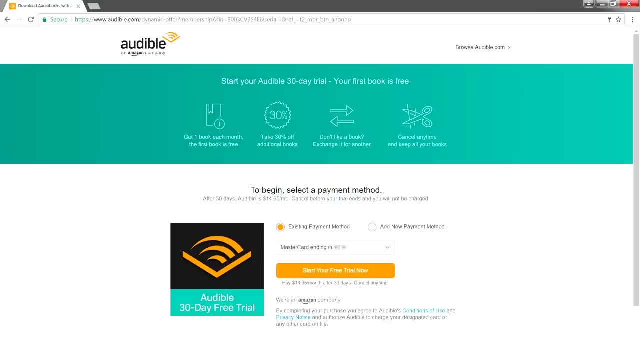 their free 30-day trial by visiting audiblecom slash afrotechmods. Once you're there, you can log in with your existing Amazon account. You need to give them a credit card number, but you can cancel your free trial at any time and you still get to keep the free audiobook. 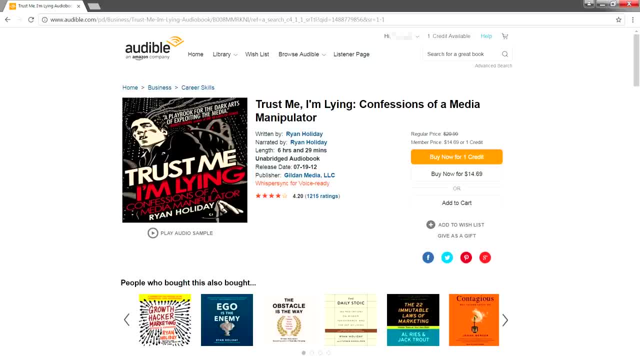 I personally like Ryan Holiday. He's got this amazing book called Trust Me, I'm Lying- Confessions of a Media Manipulator. He's got these crazy stories about how anyone can pose as a fake expert and get quoted in news articles Once you pick out your free audiobook. 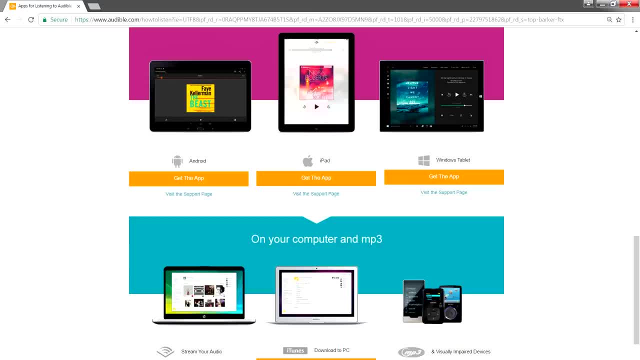 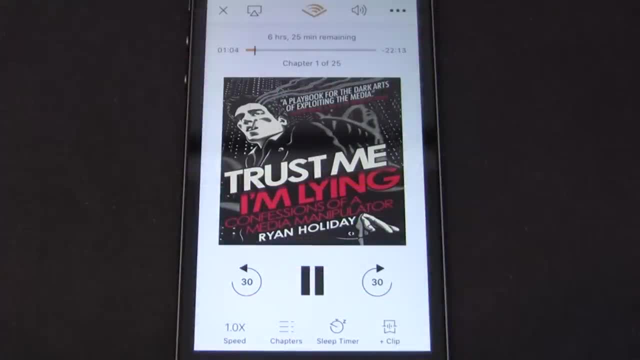 you download the Audible app on your phone or tablet and you can access your audiobooks from anywhere. I have flown bloggers across the country, boosted their revenue by buying traffic written their stories for them- fabricated, elaborate ruses to capture their attention. 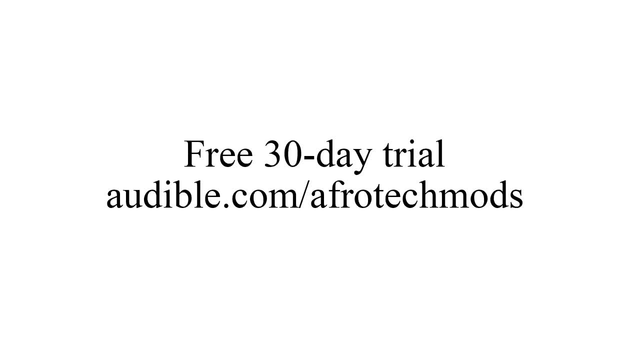 and courted them with expensive meals and scoops. If that sounds interesting to you, click on the link in the video description section or visit audiblecom. slash afrotechmods to start your free trial.